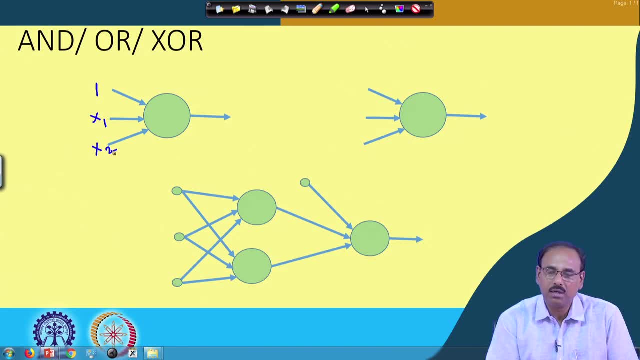 additional component, which is equal to 1.. And this is what helps in giving a bias to the neural network, or every nodes in the neural network, And the weights that we considered was minus 1.5,, 1 and 1 and with this we have seen in: 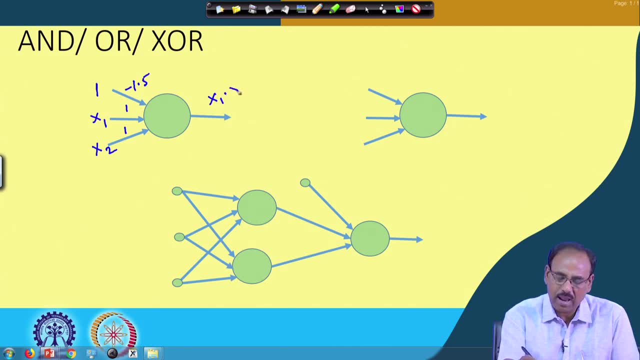 the previous class. So we have seen that in case of an AND function, if the input is X, that output becomes X1 and X2, and that is what our AND function. In case of an OR function, of course there was a non-linearity involved in it. The non-linearity. 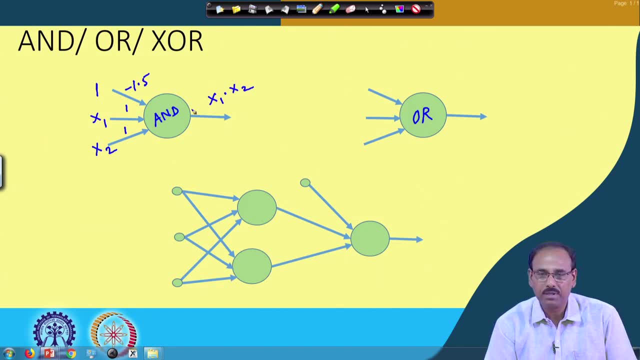 that we have considered was a threshold non-linearity. That means if the output or weighted sum of the input, that is, W transpose X, this was greater than or equal to 0. So we have assumed the output to be 1 and if it is less than 0, we have assumed the 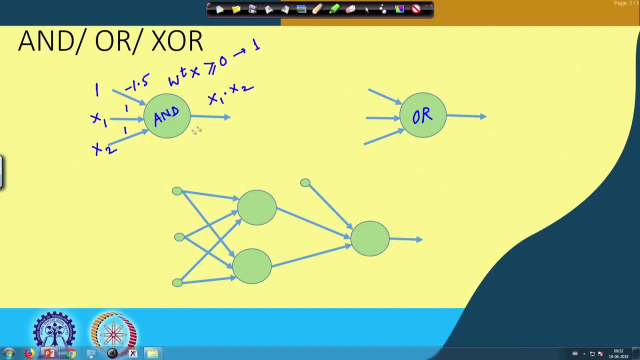 output to be 0. And with that we have seen that this network, this simple node, implements an AND function. Similarly, in case of OR function, again our input is the binary input, X1 and X2.. The bias term in this case is minus 0.5, here we have. 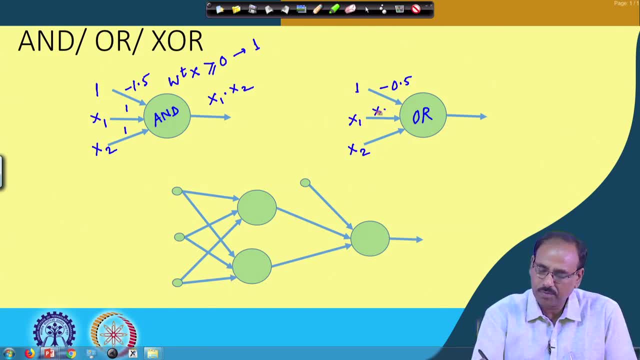 giventhe weights as 1 and 1 and with this again we have seen that the output becomes X1 or X2.. We could implement this AND function and OR function using a single neural network, because we have seen before that these functions are actually linear functions. 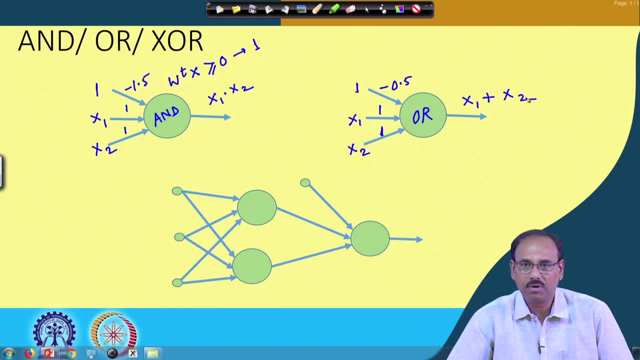 I can separate the outputs which are 1s from the outputs which are 0s by a straight line, which is not possible in case of an XOR gate. So XOR is a non-linear function and we have seen in the previous class that because XOR is a non-linear function, so it cannot be. 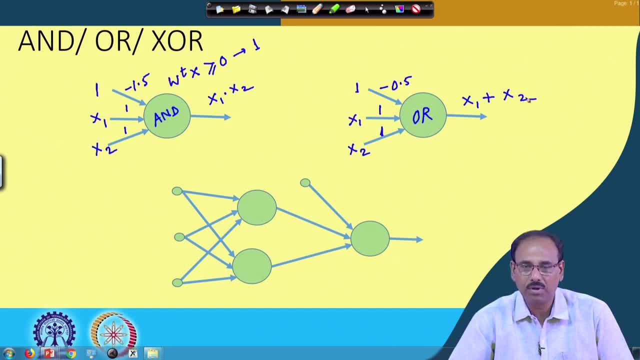 implemented a single neural network or single neuron. So I need multi-layer neural network and that is what is required In this figure. So here again, our inputs are 1, X1 and X2, those are the binary inputs. And one of these two gates we have seen before that it implements an OR gate and the other 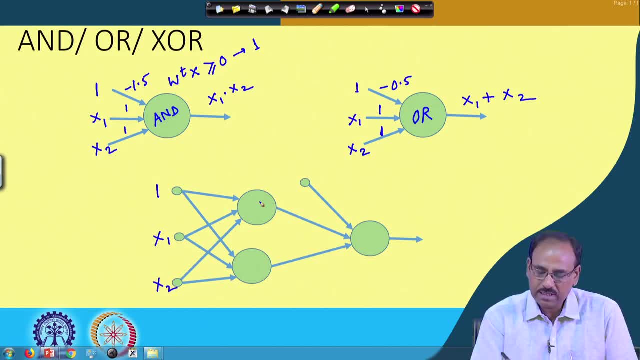 one implements a NAND function. So let us assume that the first one implements an OR function and this one implements a NAND function. So for implementing OR function, just as we have seen over here, our weights will be minus 0.5, 1 and 1, and for implementing a NAND function, it has to be just complement. 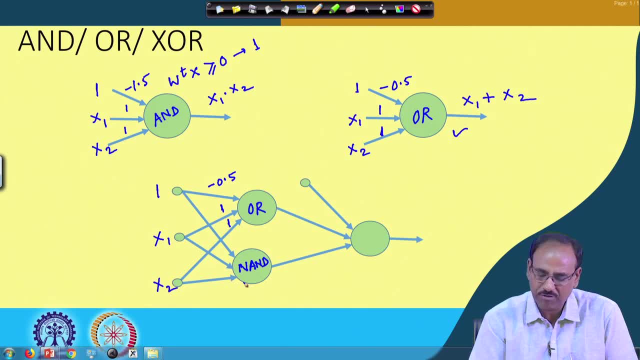 of AND. So weights for implementing NAND function will be plus 1.5, minus 1 and minus 1.. And these two outputs are finally to be ANDed, Because OR XOR function, X1, XOR, X2 is nothing but X1, or X2 ANDed with X1, NAND, X2. So here, 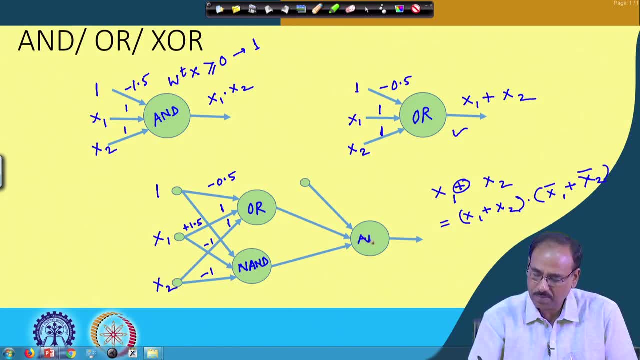 I have to have a AND function. So for this weights will be minus 1, 1, 1, and 2. So we have a AND function. So for this weights will be minus 1, 1 and 1 and minus 1 and minus 1 and minus 1.. So 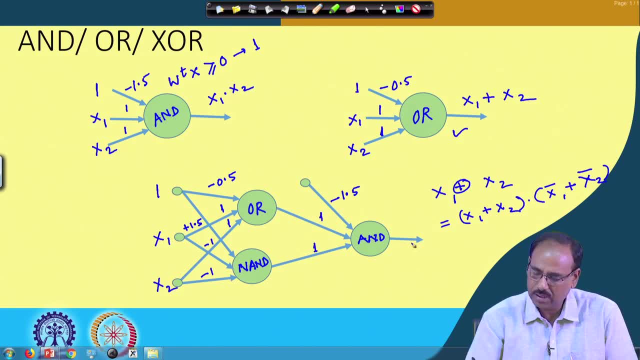 1.5, 1 and 1.. So here at the output, what I get is x, 1, x or x, 2.. So you find that these are simple implementations of the logic functions usingneural networks. Now from: 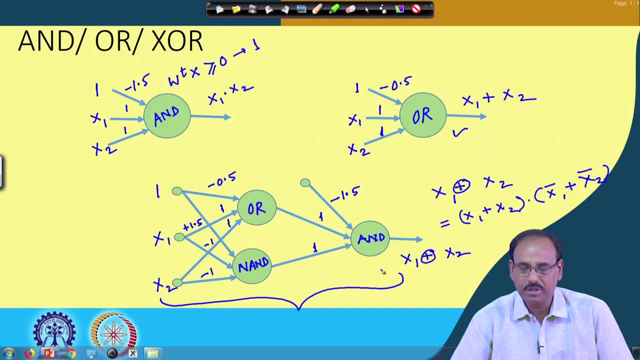 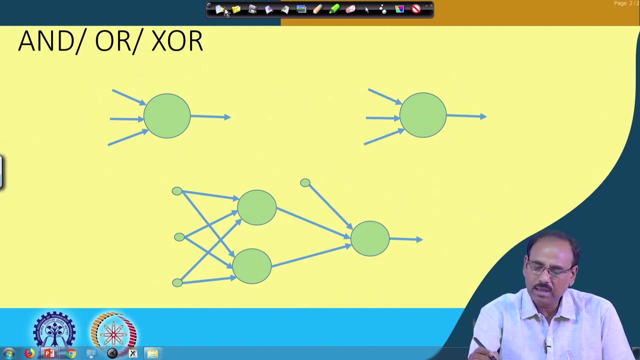 particularly this XOR function. it is quite obvious that if the function that we have to implement or the problem is a non-linear problem, the non-linear problem cannot be solved using a single layer network. I need multiple or multilayer neural network for implementing a non-linear problem. So for a non-linear problem, as we also have, 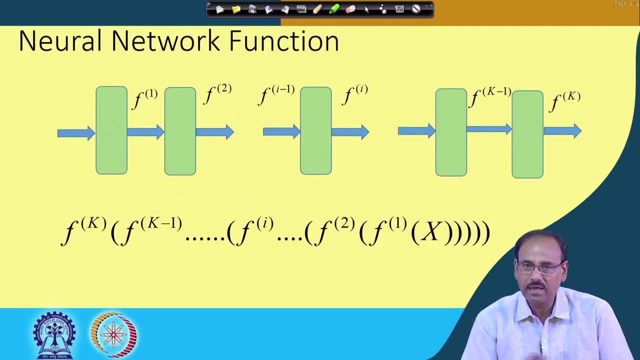 seen in the previous class that I have layers of neural networks. So I have neural networks in multiple layers And we have also that there are multiple layers of neural networks, layers, and from every layer- say layer 1 to layer 2- I havecomplete connection. that is. 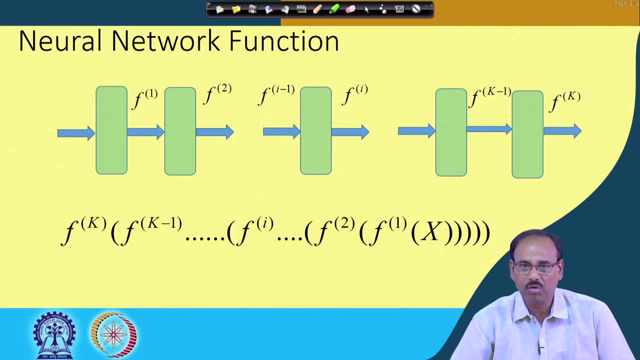 every node in the layer 1 is connected to every node in the layer 2 and if the final function, So here you find that there there are k number of layers. So at the output I call the output layer to be kth layer. So the final function that is being implemented. 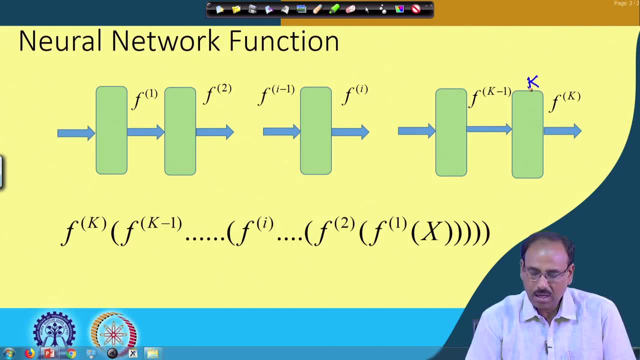 is f k, ok, and the input layer implements a function f 1.. So, with my input vector at as x, the first layer, that is, f 1 layer, it implements function f 1 of x. the second layer implements f 2 of f 1 x. third layer will implement f 3 of f, 2 of f 1, x. and finally, 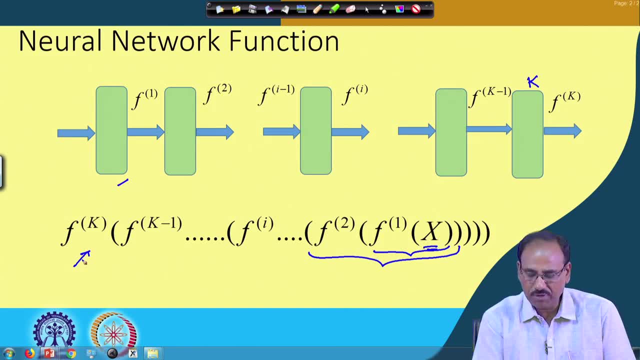 the kth layer implements f 1 of f 2 of f 1 x. So it implements f k of the output that has been generated by all the previous layers. So when it is a non-linear problem we can say that all the layers from f 1 to f k minus. 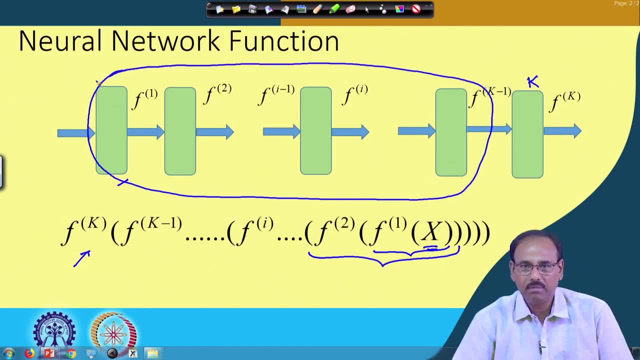 1, they will implement a non-linear mapping Because, as we said earlier that if I have a non-linear problem, then instead of trying to design a non-linear classifier, you would try to map the input vectors using a non-linear mapping function So that they are mapped. 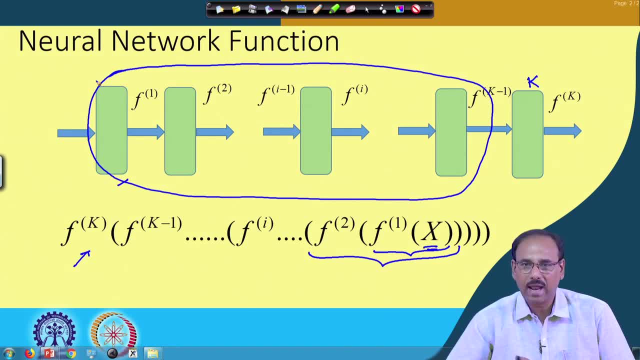 intointermediate feature space, and in the intermediate feature space this non-linearly mapped input vectors will be linearly separable. And then finally, at the final layer or at the kth layer, I can have a linear classifier to classify all those samples correctly. So 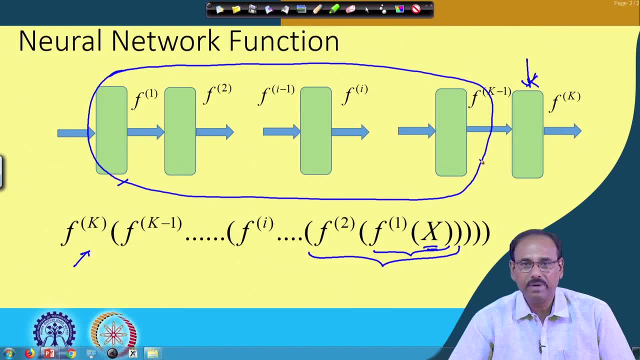 all these layers, from f 1 to f k. they actually implement this non-linear mapping function. So at the output of f k- the new feature vectors that I get a feature vectors x, which are now linearly separable, and the kth layer- I can implement a linear classifier which 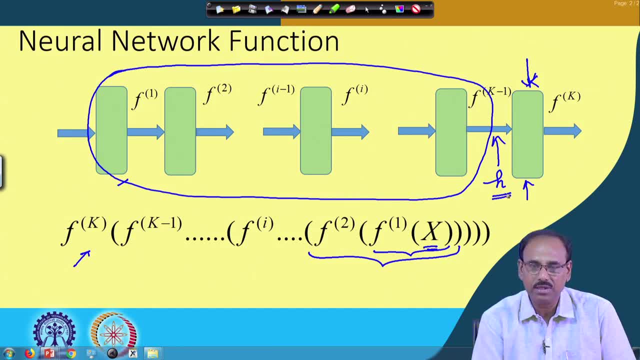 will classify all these vectors h which are now linearly separable. So this is just a block diagram representation of a multi layer perceptron or a fitted Vegatron. So in the case this the vector is not directly separated from the vector line, So from this an implicit 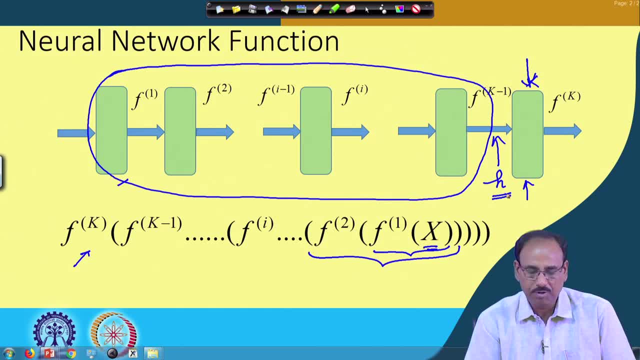 vector we can create a linear vector. So with the extra vector I can implement the forward neural network. Now why it is feed forward? Because I am inputting the feature vector x at the input layer. they are being processed at every layer. 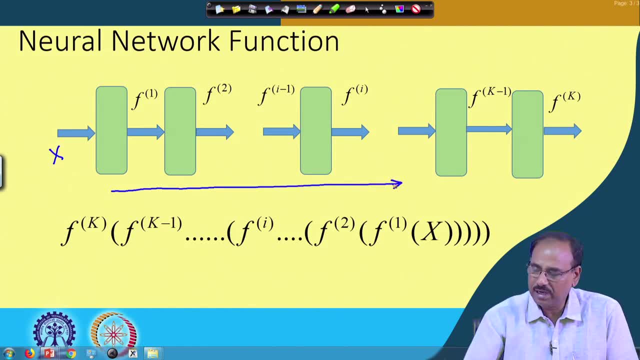 and being forwarded in the forward direction to the next layer and finally you get the output from the final layer at the output layer And nowhere in this path the information is fed back to the previous layer. So always the information flows in the forward direction. 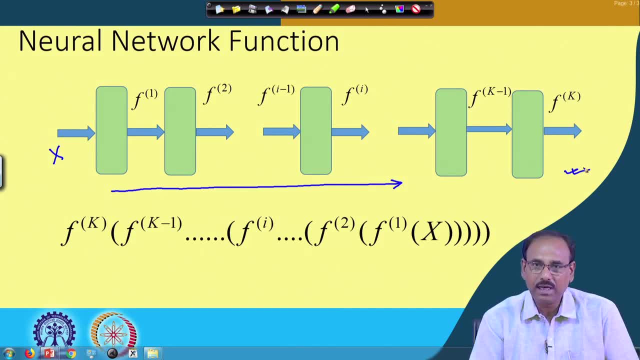 so it is feed forward network. But we will see later that for learning or for training this neural network, the error is propagated in the backward direction, Because our aim is to minimize the error by adjusting the weights in between the layers. So for training, 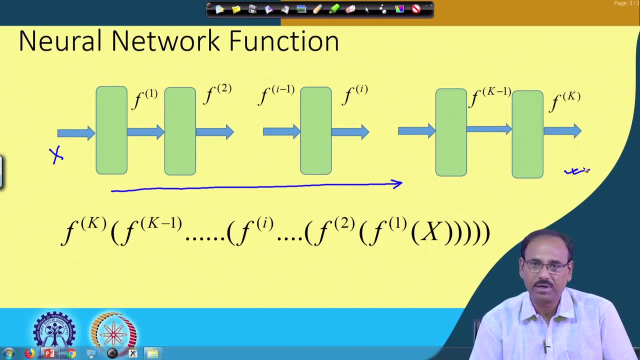 this neural network, the error is propagated in the backward direction through each of the layers, and while it is being propagated at every layer, the weights are updated to each one in order to minimize the errors. So that is why the learning algorithm is known as back propagation learning. So our neural network is a feed forward neural network. 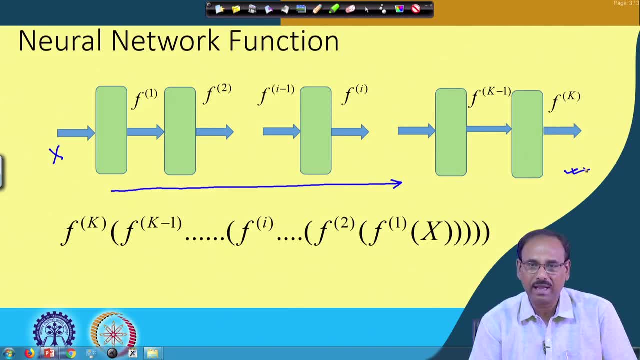 but the learning algorithm is a back propagat, is a back propagation learning algorithm. Now let us see in details that this, how this neural network or multi-layer perceptron that looks like. So we will now start to understand that And clearly that is definitely. not the early days theory. Now let us look at that general idea before I finish青 skill. Now take advantage of the self �est way first, that we can understand how similar or inverse this neural network is played overöl by shrink embedding attacks, mainly Franco and Haygons, And I am. 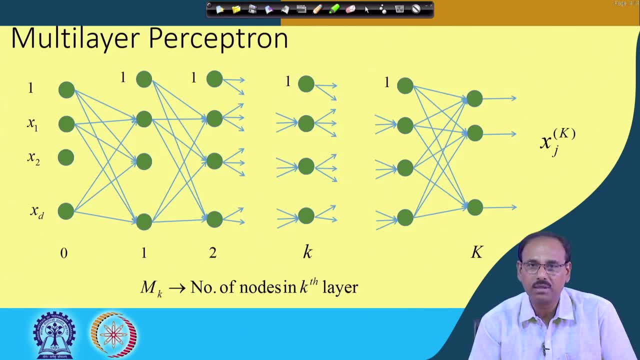 So this is what is a somewhat detailed representation of the speed forward neural network. So here I have assumed that there are k number of layers in the network. At the beginning we have an input layer which is represented as zeroth layer. The purpose of this layer is: 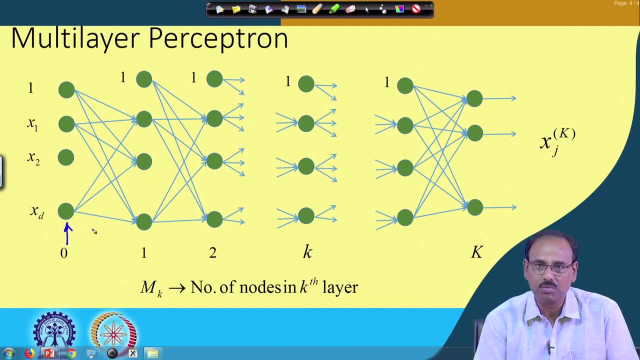 simply, whatever comes at the input is simply passes to the output. So this layer does not have any other function other than simply passing the input to the output And every other layer, from 1 to say layer k minus 1, each of these layers participate. 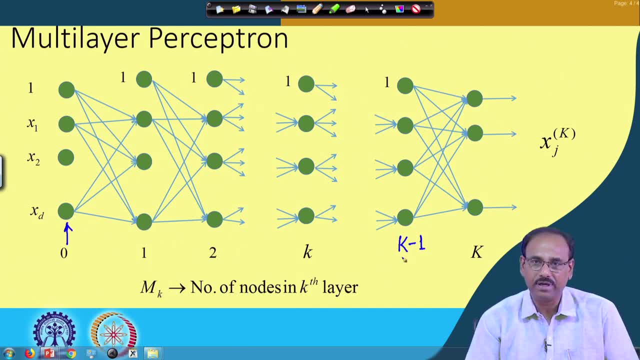 in non-linearly mapping the input feature vector x to a new feature, space H And k-th layer, which is represented by capital K. it is the final output layer, right, And we also assume that k is the output layer. So k is the output layer and k is the output layer. 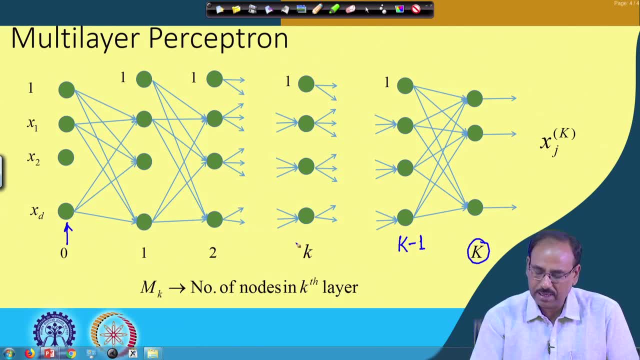 So we assume that from every layer, every intermediate layer k, where this k is represented by lower case letter, the nodes are connected or the neurons are connected to the next layer, which is k plus 1. And this connection is complete in the sense that every node in the 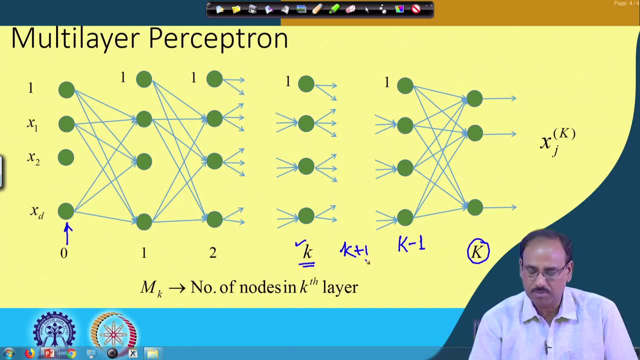 k-th layer is connected to every node in the k plus 1 layer And if I take an ith node in the k-th layer, It is connected to j-th node in the k plus 1st layer through. So let me put it like: 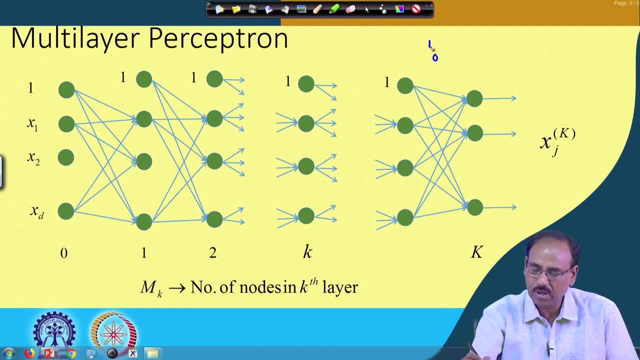 this. So I take a node i or a neuron i in the k-th layer and I take a neuron j in the k plus 1st layer, which is the next layer. So the output from the node i is connected to the input of node j. Output from node i in k-th layer is connected. 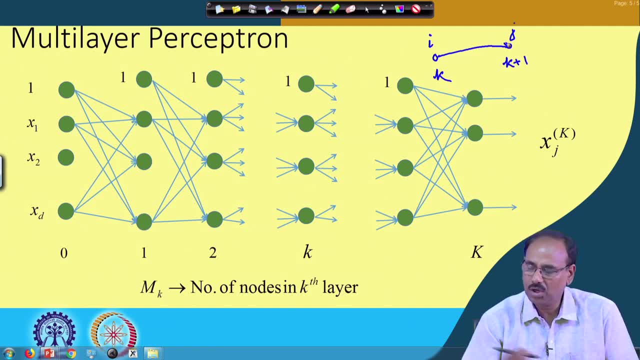 to the input of k-th, because first layer through a connection weight which is w, i, j, k plus 1.. So this is the convention that we will use when we discuss about the back propagation learning. So this is the overall architecture of our 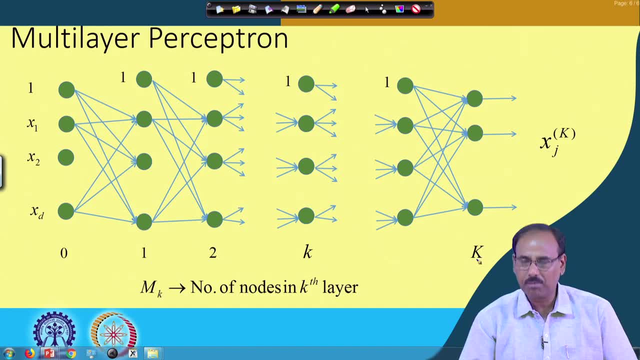 feed forward nasal network. There are k number of layers. k-th layer is the final output layer. Every node or every neuron i in an intermediate layer k, represented by lowercase k, is connected to the nextconnected to the jth node in the k plus first layer through an weight which: 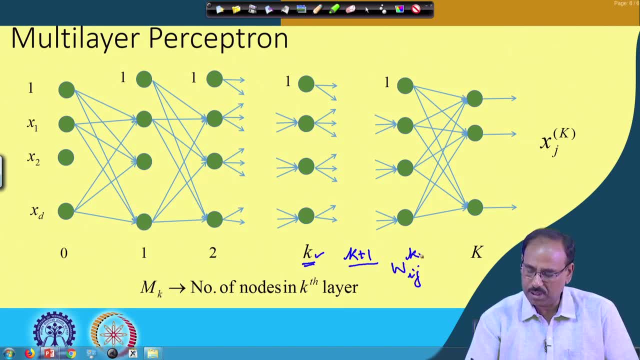 is given by W, ij, k plus 1.. And the purpose of training this neural network, or learning, is that iteratively, using the training vectors, you try to find out what should be the value of W, ij, k plus 1 for every i, j and k, so that the neural network is finally. 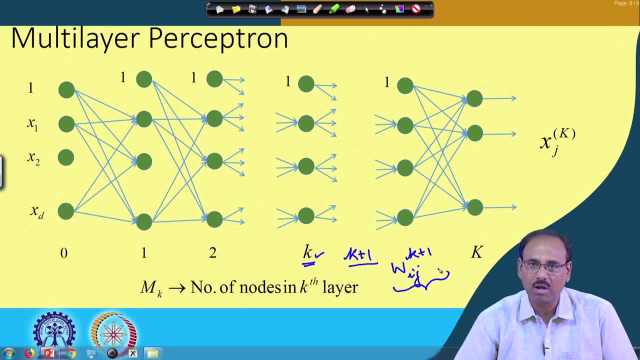 trained to solve your problem. So that is the purpose of back propagation neural network. And in this network you find that as we are feeding the input x, i, So for training we have the training data is fed in the form of x, i, y, i, as a doublet for, say i is equal. 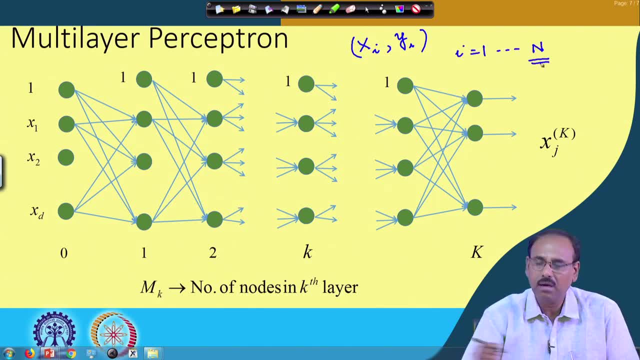 to 1 to n, where n is the number of training samples I have which is given for training this neural network. So for every training sample, x, i as it is labeled, because these are used for the training purpose, I know that to which class the training. 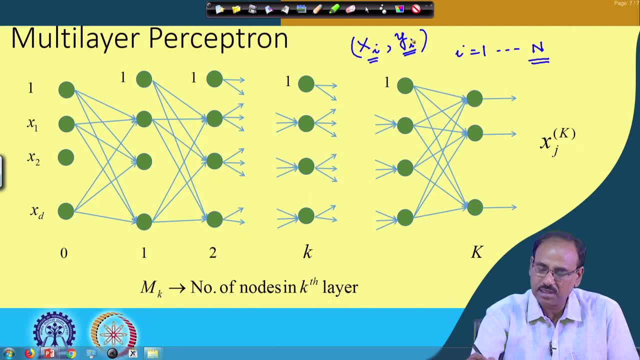 this sample x i belongs, So x i in this case belongs to class y i. So if I have a binary classification problem, we will do thatquickly. this y i can be either 0 or 1.. If y i is 0, 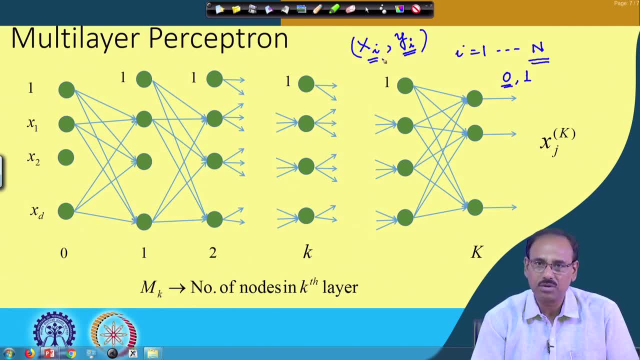 that means the sample x i belongs, to say class 1, omega 1.. And if y i is 1, that means the same: the sample x i belongs to class omega 2.. So this tells you that what is the class belongingness of the training sample that I have. 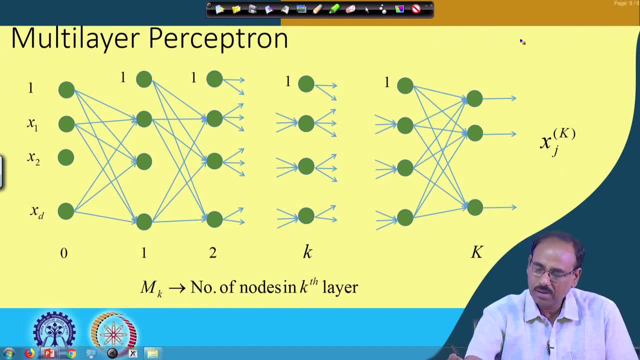 If I have c number of classes. if I have c number of classes, then y i will take one of the values 1 to c. So this y i in that case is the index to the class to which x i belongs. So if I have a data x i, 5, this is the training data given, then this means that the training 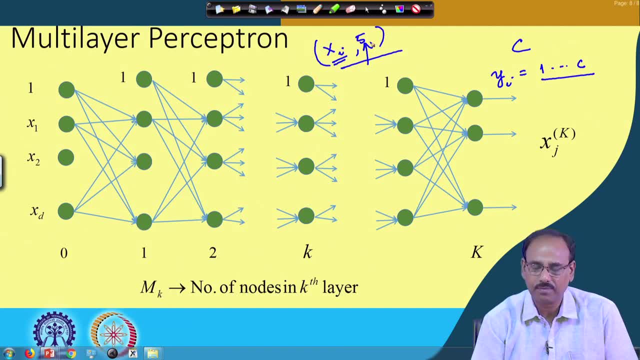 data x i belongs to class 5.. Secondly, at the output node. if I take a j th node, j th column at the output layer, I represent the output of the j th node in the k th layer as x j k. So these are the conventions that we will use when we talk about back propagation. 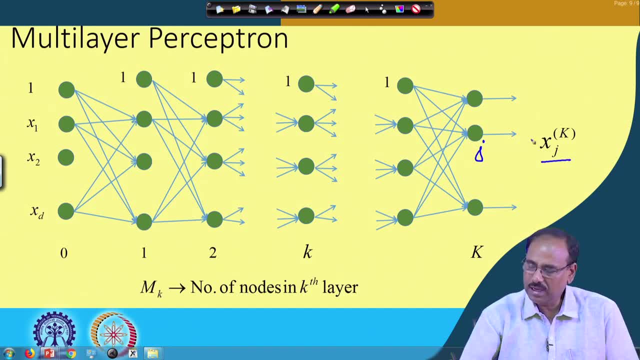 learning. And here you find that only at the output given attaining vector x i. only I know that what should be the corresponding output? Because if it is x i, 2. This is the training pair that is given. I know that when this x i is fed to the input, 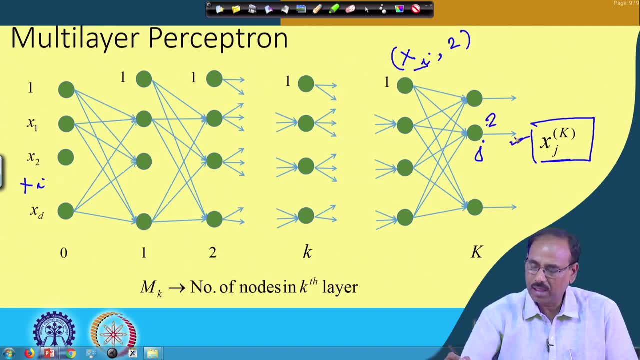 output of the second node. that should be high. the outputs of all other nodes should be equal to 0.. Because my training pair says that this vector x i belongs to class 2.. Similarly, if attaining vector x is given, which belongs to class 9, then when I feed this x i to the 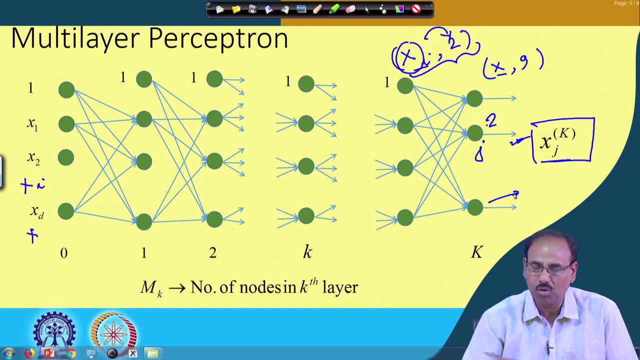 input only the output of the 9 th node from the output layer should be high and all other output should be low. So this I can decide only at the output layer. I really do not know that. what should be outputs of any of the hidden layers. that is not visible. So 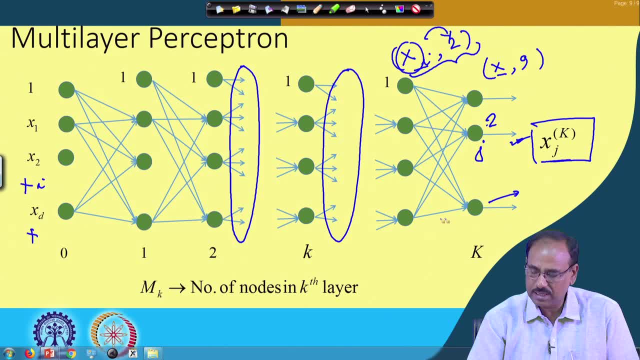 that is the reason that all the nodes or all the layers, except the output layer, they are known as hidden layers, Because I can only observe. I can only observe, only decide at the output. I cannot decide what should be the outputs of any node in. 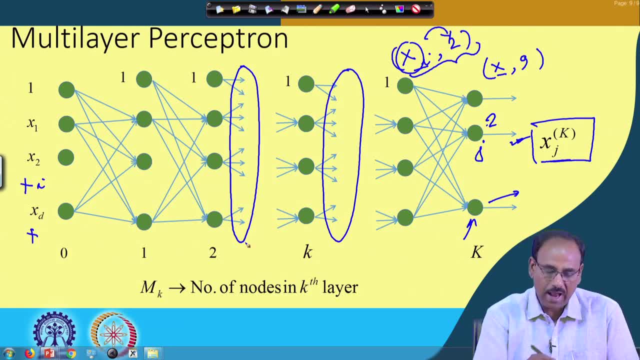 the intermediate layers or hidden layers, And this is a layer, as we said that this is known as input layer. So the purpose of every neuron in the input layer is simply to pass whatever is coming to the input to its output, and it is subsequently fed to the neurons. 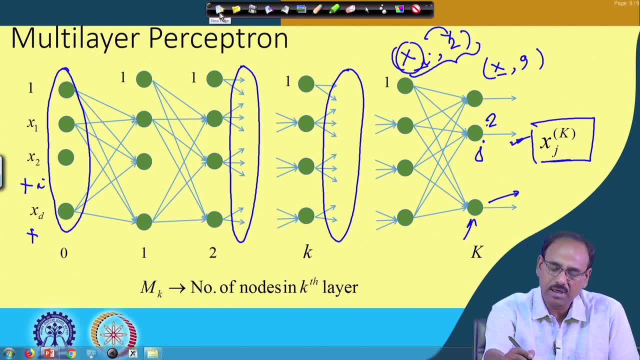 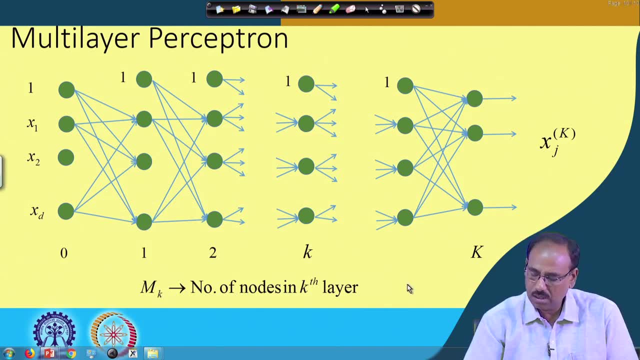 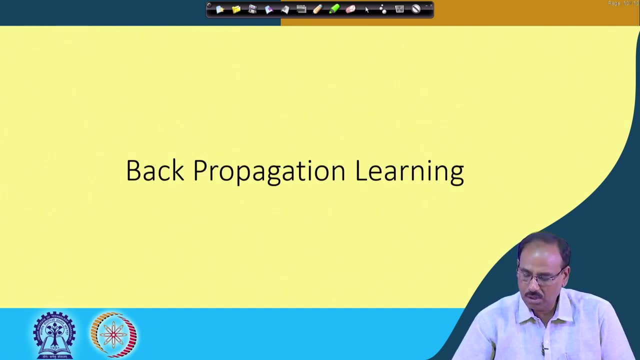 of the next layer. So this is what the architecture of the neural network looks like And the conventions that will follow. Now let us see that. how can we train the neural network, or what is back propagation learning? So to talk about back propagation learning, 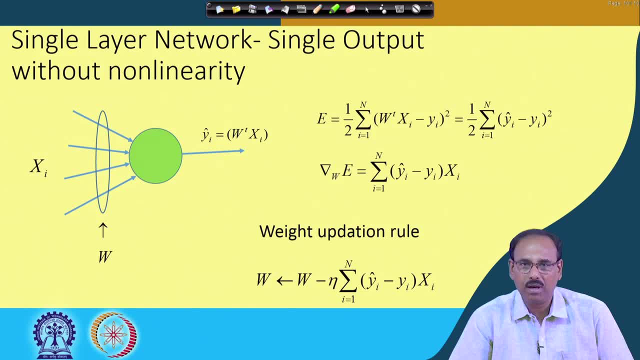 first I will consider a very simpleneural network consisting of a single layer, which is the output layer. Of course you remember that we said before that using So back propagation. This is the output layer And you will be able to a single layer. I can solve only linear problems. I cannot solve any non-linear problem. 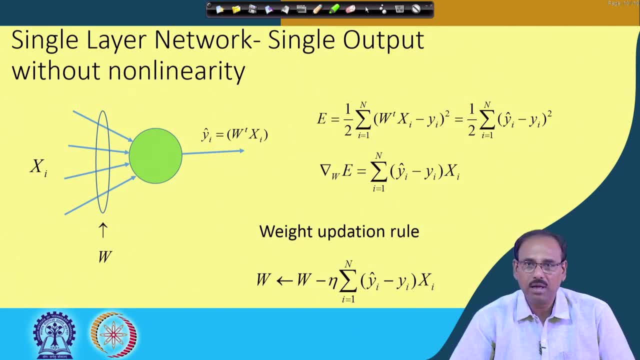 And, as I said, that this learning algorithms will do in details, because this forms the basis of all subsequent deep learning or deep networks, deep neural networks that we will talk about. So it is very important that you understand the back propagation learning very, very clearly, right? So again, I take a single network, a single 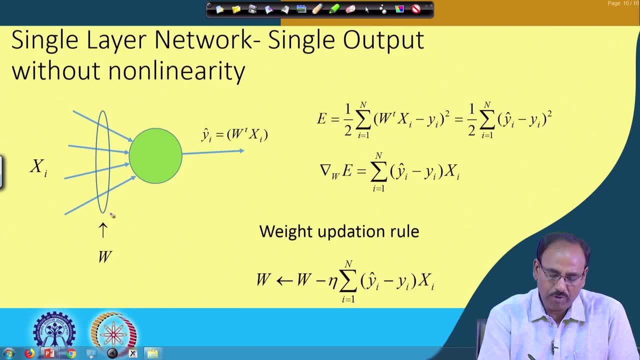 neuron where the weight vector is w, if I feed an input vector x i. So, as we said before that for training I get the input vectors as pairs x, i, y i, where this y i is the class index to which This vector x i belongs, and, as we said, that this is used only for training purpose during. 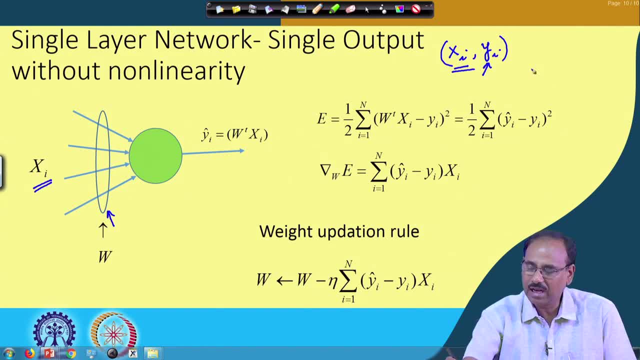 actual testing or when you deploy such neural network. I have an unknown vector x. I do not know what is the y. if I know, then I do not have to classify that and that classification will be done by the neural network only. So here, as I have or as I feed such an input, vector x i, I expect that the output of the neural network will be what? So I have a injection vector where X- i will be Japanese, And I want to have all vectors in the neural network. where X, i, this vector x belongs, ast counted. that means thisence only because, if I anything, I homemade these super cont besoin. 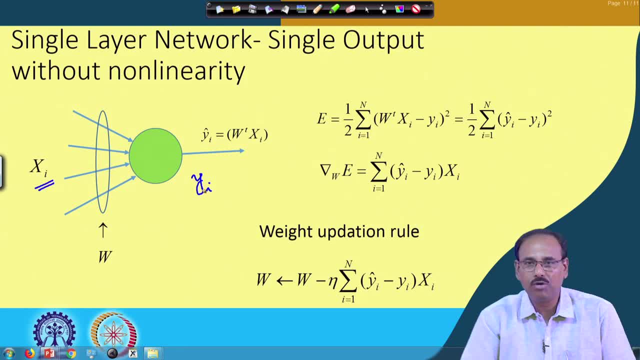 of such. So what I did is, if I deployed such an input, vector x, i, I expect virtual 마스� Saltz weapon output of the named neural network I, which means that the space network should be y, i, and only when I get the output as y, i, which matches with mytrue. 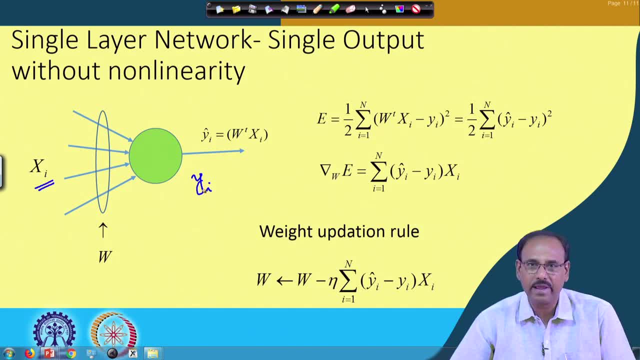 values, then at least this x i is correctly classified by this neuron. But what we get is: I get a value x i hat which is an approximation of x i. So if x i hat, so this x i hat is nothing but w. transpose x i, where w is my weight vector and x i is the input vector. 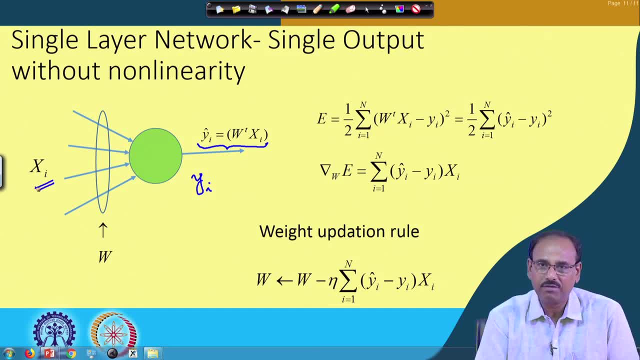 And for the time being, I am assuming that I have a neural network with single layer and single output node and I am not assuming there is any nonlinearity in this neuron. ok, So my output simply becomes w transpose x- i, and I am assuming that this w transpose 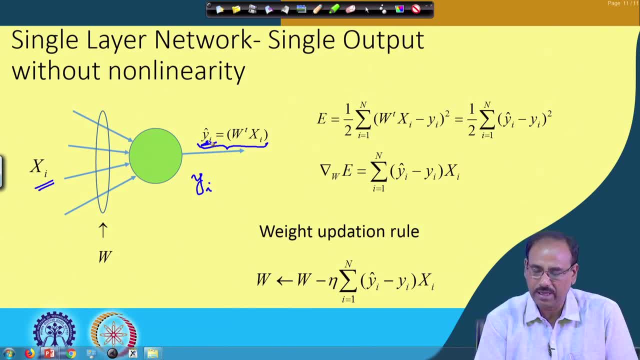 x i is an approximation of x i, So I get an approximation to y i which is y i hat. So if y i and y i hat they are same, that means my input vector is correctly classified So I do not have to take any action to modify. 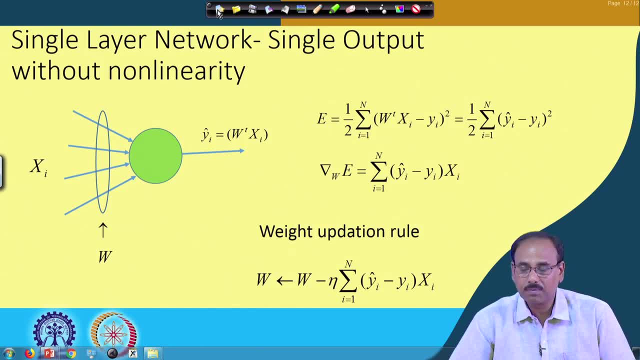 the weight vector w. Now suppose y i hat and y i. they are not same, they are different. ok, So my error will be y hat minus y i. this is the error, And what I compute is the sum of squared error. So this is sum of y i minus x i, where this i will vary from. 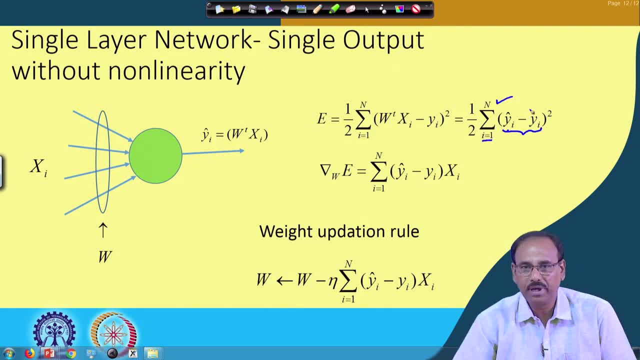 0 to n. So this squared error is computed over all the training vectors that I have, as i varying from 0 to capital N, And I have capital num, capital N, number of vectors for training purpose And I scaled it, this by half. the reason of scaling it by half is: as we have seen earlier also. 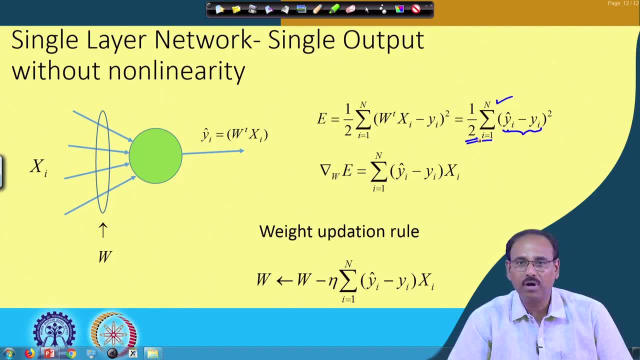 Okay. So for any learning algorithm or any training algorithm, we go for gradient descent approach. that means I have to take differentiation of the error function or the loss function that we have generated, And because it is squared error or squared loss, 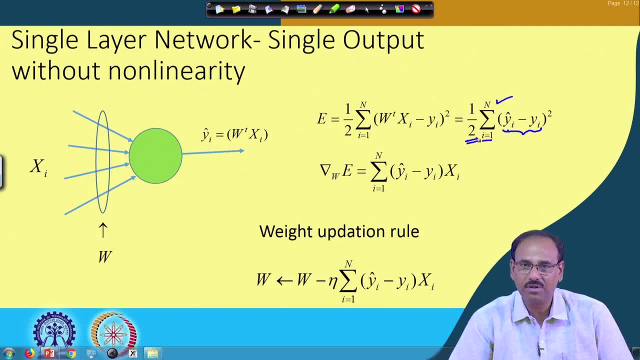 So having a factor half will simplify our expressions. So that is the reason this half is put, if I put it in an elaborated form. So this error function or the loss function e is nothing but half of W. transpose x: i. 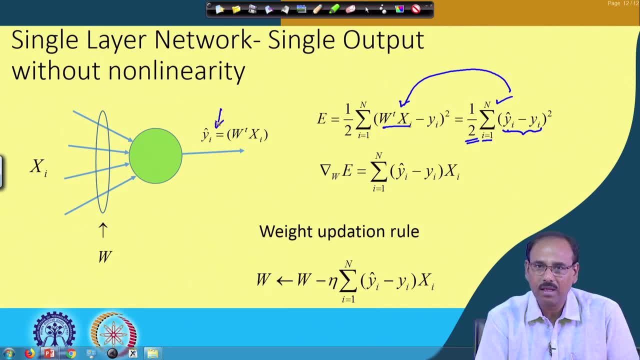 this: W transpose x, i is nothing but our y hat. So W transpose x, i minus y, i squared. take the summation over all i varying from i equal to 1 to n. that means you are summing the errors of all the training vectors that you have. 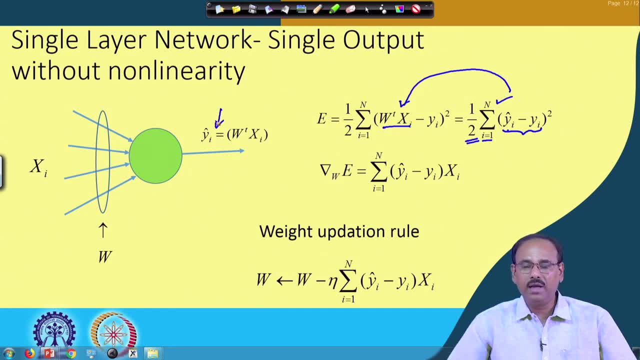 Next, as we said that we will employ the gradient descent approach, as we have done before for training the network or for updating the weight vector W. So I take the gradient of e with respect to weight vector W, and here you find that this gradient is nothing but y hat minus. 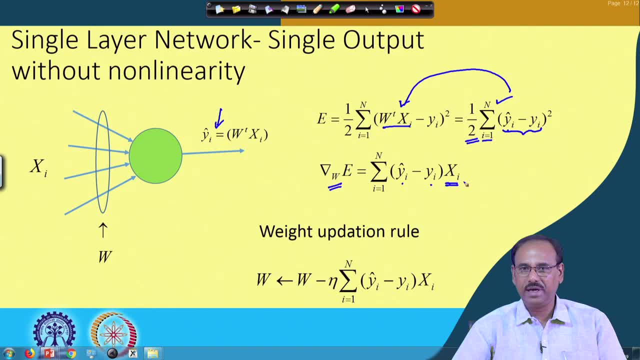 y i into x i, where x i is the input training vector right. And now you find that why we have put this half, because otherwise there would have been a scaling function 2 over herescaling factor 2 over here. So in order to avoid that you put half. So this is the gradient of the error or the loss. 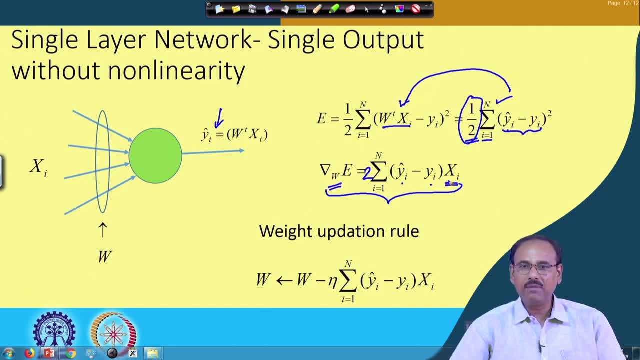 right. So I have to update W or the weight vector in such a way that this loss is minimized or the error is minimized, And for that, as before, my weight updation rule follows the gradient descent procedure, So my weight updation rule will be simply. 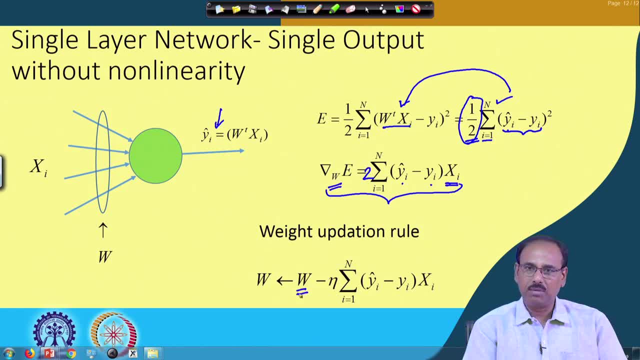 W gets. if this is the previous value of the weight vector, the updated weight vector will be W minus some eta times the gradient. What is this eta? We also said before that this is nothing but a rate of convergence factor. So this eta indicates if the value of eta. 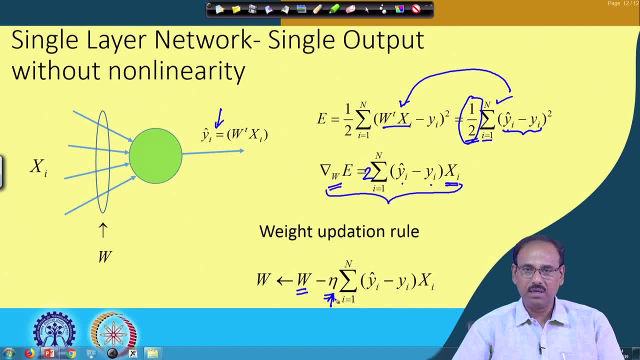 is very high, then the rate of convergence will be fast. if the value of eta is low, then the rate of convergence will be low, So I will have a slower convergence. of course both has their individual merits and demerits. we also discussed about those before. Now, if you look at this weight updation rule, 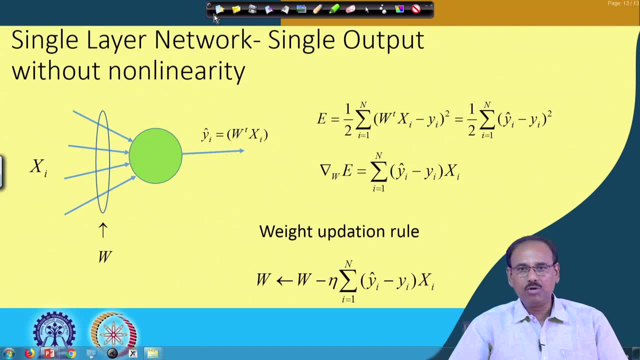 you find that we get something more. I said my output Y should be either 0 or plus 1.. So if it is 0, it belongs to one class, if it is plus 1 it belongs to another class. And if you remember that earlier, the linear discriminators that we have talked about, 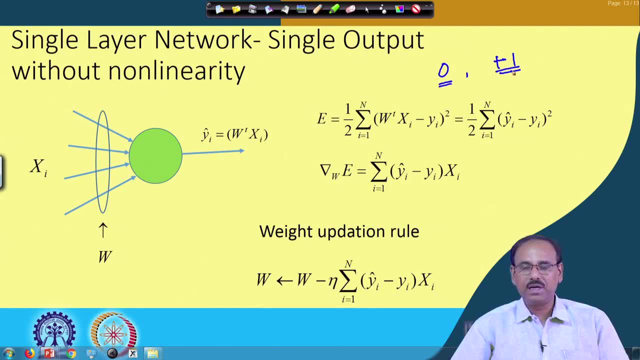 that is, a linear plane which separates two different classes which are linearly separable. We have said for one of them: if W transpose X greater than 0, then it belongs to one class, if it is less than 0, it belongs to one another class. Now here let us come to a situation. 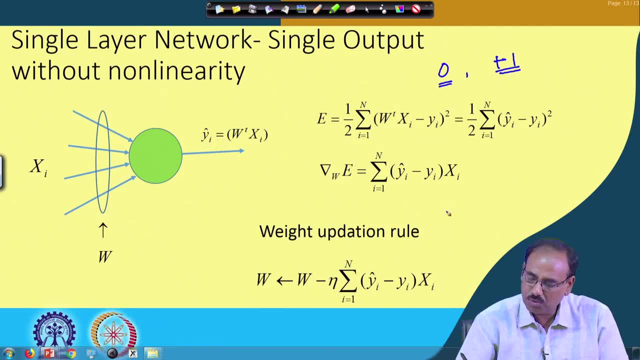 that. So if I find that W transpose X is greater than 0 for samples belonging to some class omega 1, and this is represented by Y, i is equal to plus 1.. So as long as my W transpose x i is greater than 0, then it is correctly classified. right Now here you find that. 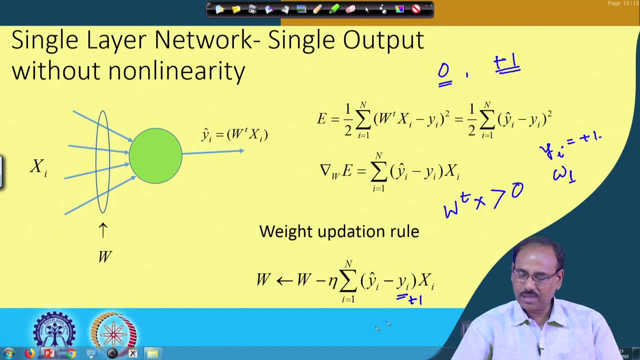 if my Y i is plus 1, but I get the Y i hat to be negative. Then, and instead of taking the sum, let us consider a single feature, vector X, i So, which is nothing but stochastic optimization. talked about that before. If you sum all of them, that means you are considering all the. 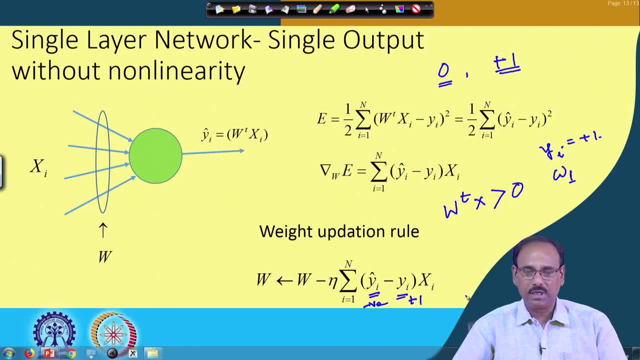 training vectors. together it becomes a batch optimization technique. So we have talked about batch optimization, mini, mini batch optimization and stochastic optimization. So if I consider only X, i, that becomes a stochastic optimization procedure and then our weight updation rule will be simply: W gets W minus eta times. Y i hat minus Y i times. 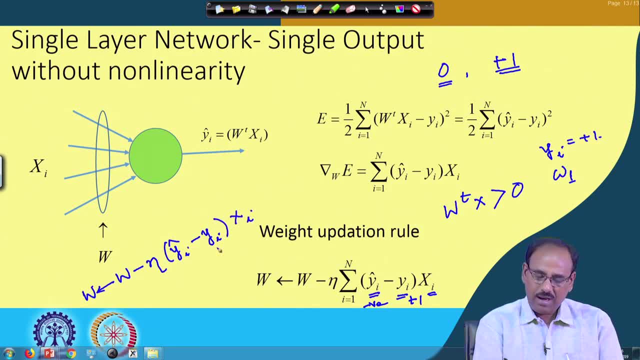 X i. So here, if my Y i is actually plus 1, that means W transpose X should be greater than 0 for correct classification of X i. But suppose W transpose X, which is nothing but Y i, So W transpose X should be greater than 0 for correct classification of X i. 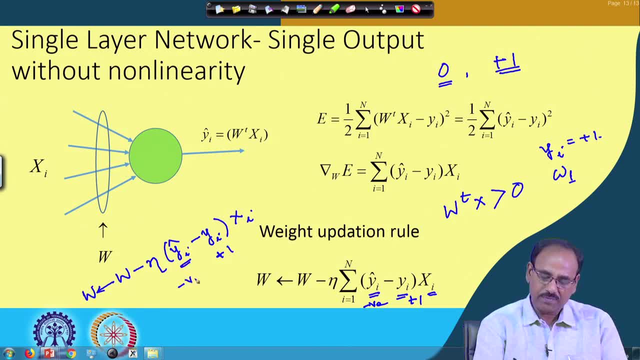 So Y i hat happens to be negative. In that case, this Y i hat minus Y i, this whole term will be negative and in effect, what we are doing is we are making W, updating W, as W plus some factor, say eta times. let us put chi times X i.